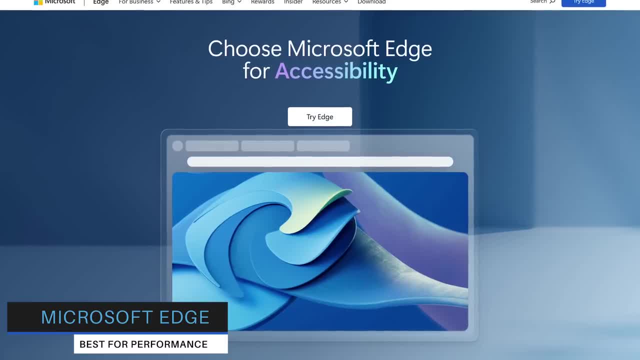 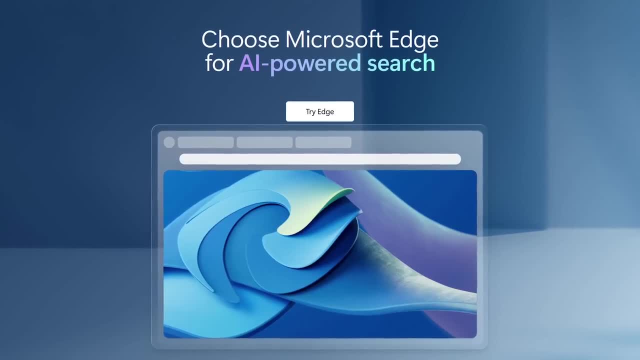 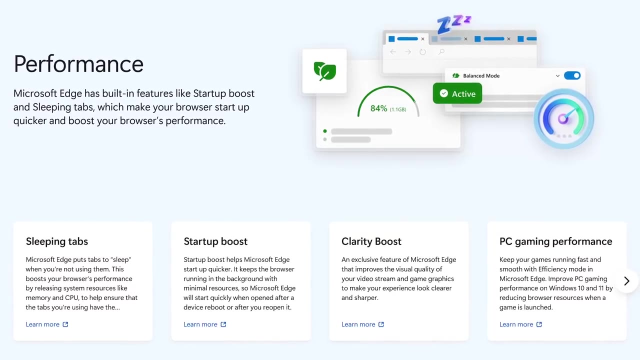 In the category Best for Performance, Microsoft Edge takes the lead. This wicked, fast browser based on Google's Chromium loads quickly and is better optimized for Windows computers than Chrome, And it even runs better on M-Series Macs than Chrome. Some of the performance features include sleeping tabs, which puts 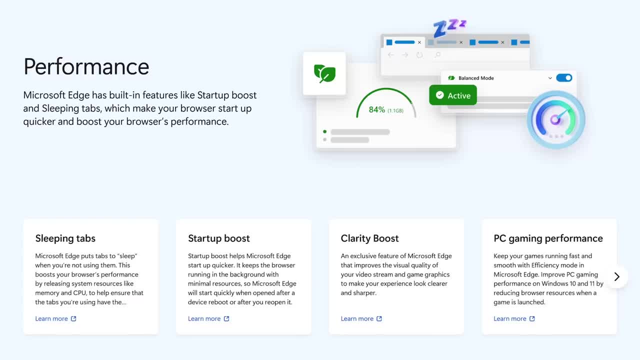 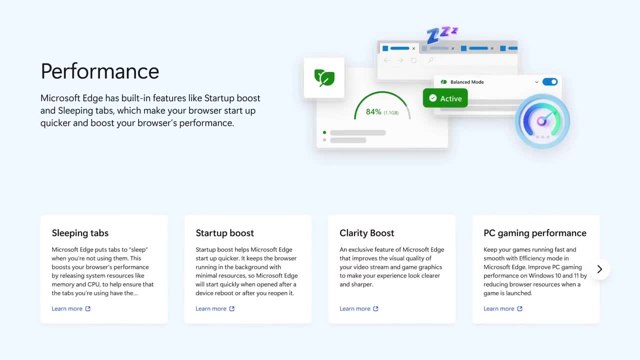 tabs to sleep when they're not in use. startup boost helps Edge to start up quickly. clarity boost makes game graphics and video streams look clearer and sharper, and there's a feature to improve gaming performance. As much as I've been trying to avoid the hype cycle with artificial 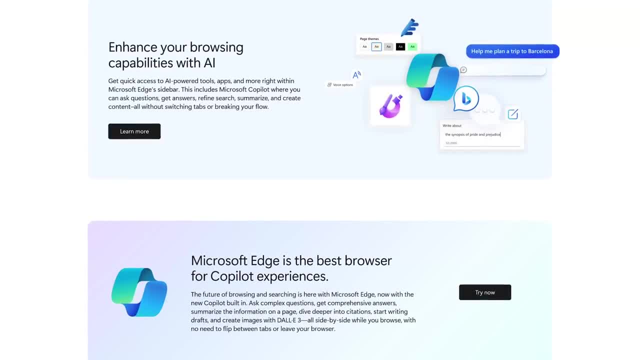 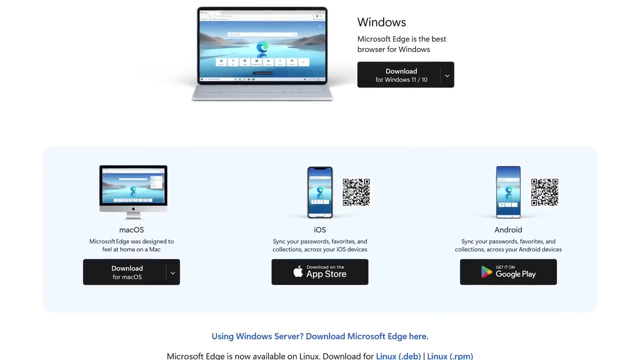 intelligence and language learning models. there's no denying that Microsoft's AI tools built into Edge has Google running scared, and that's not necessarily a bad thing. An annoyance with Edge is that it nags a lot, even more so than a typical spouse. 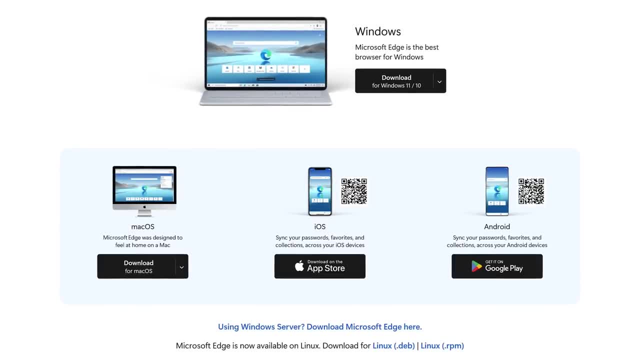 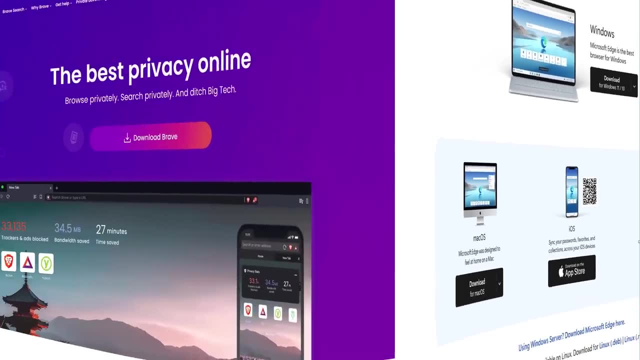 It really wants you to like it and begs to be the default browser. It's available on all the major platforms and, in a shocking move, is now available for download on Linux computers. Up next, the Brave browser is the best for privacy. 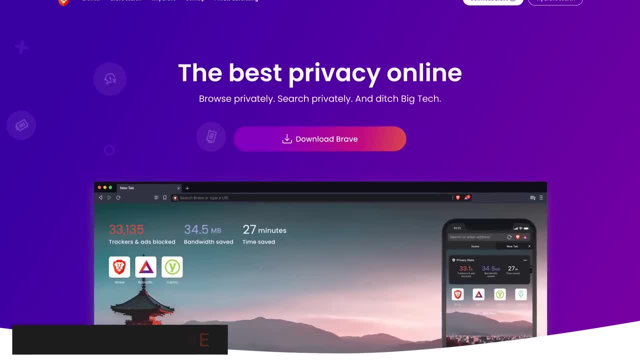 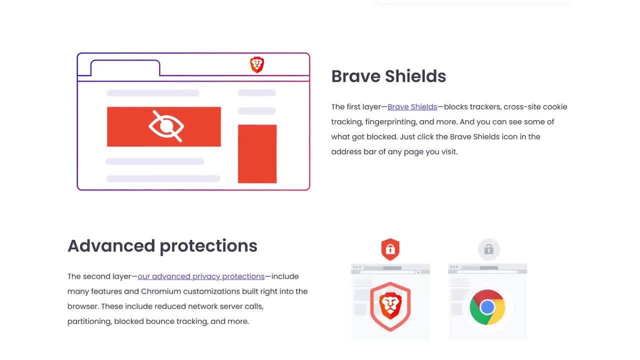 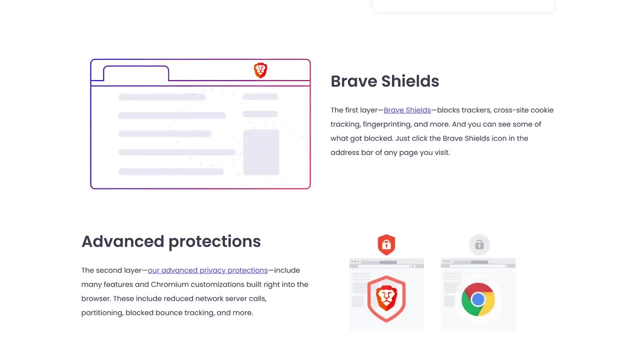 This open source browser based on Chromium, when tested by the Electronic Frontier Foundation, had the best results in their Cover Your Tracks privacy test. Its three layers of privacy are turned on by default. Its Brave Shield blocks trackers and those creepy cross-site cookies that follow you from site to site. Its advanced protections. 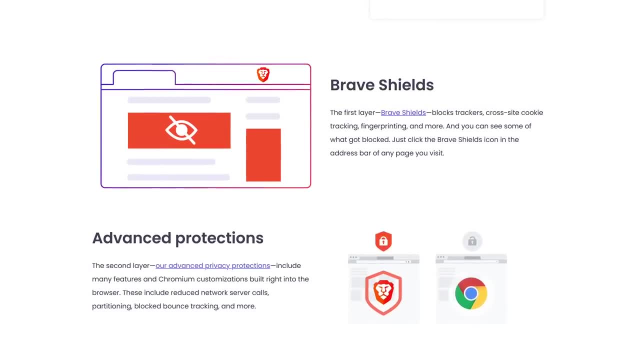 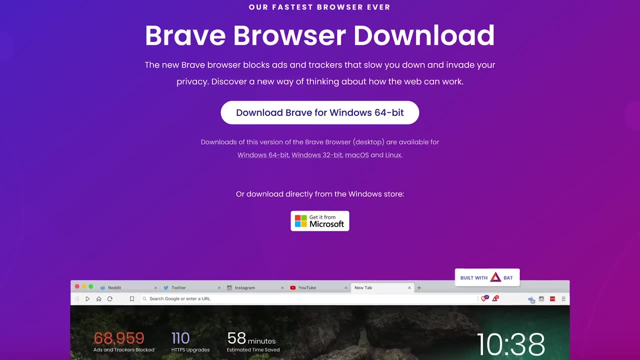 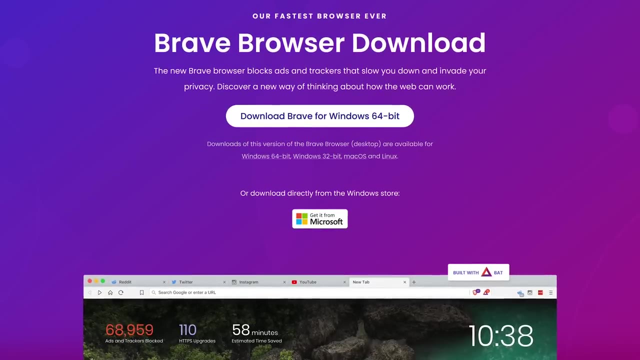 limit network connections with its backend servers and includes social media blocking, And its privacy policies and practices are quite strict. They don't even collect your data. While Brave is available on all the major platforms, a couple downsides are that it has limited support for extensions and because it blocks trackers so aggressively. 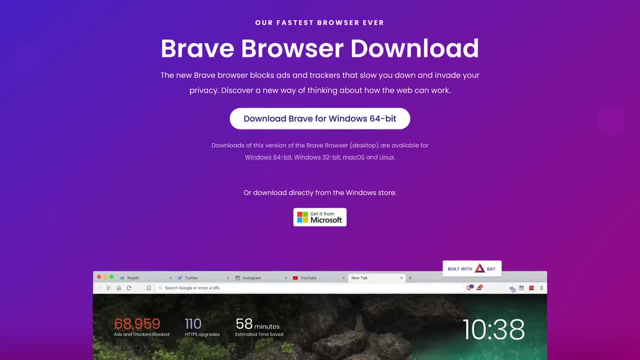 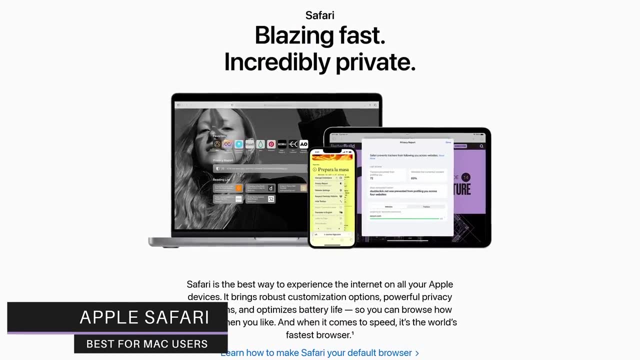 some web pages may not load properly. Other than that, it's a very good browser, Only available on Apple devices. Safari, which is the default browser on Mac and iOS, is the best browser for Apple fanatics that are hesitant to use third-party software. 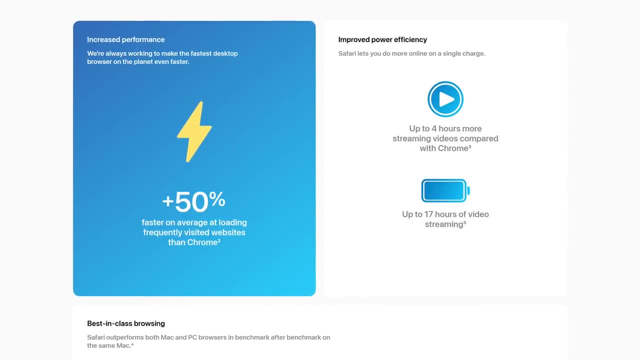 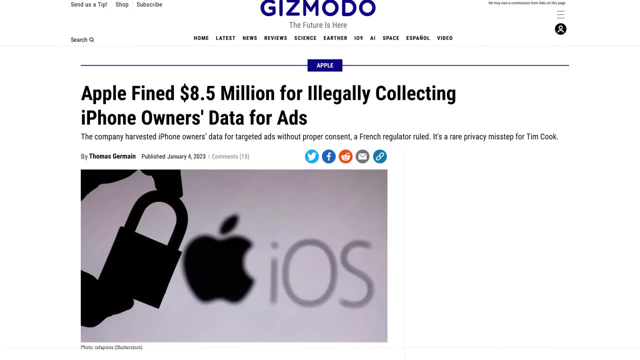 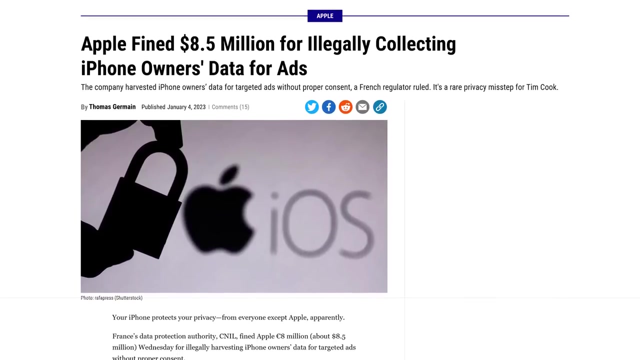 Since it's specifically designed for use with Apple devices, it's optimized to run better than other browsers with longer-lasting battery life on Apple laptops, phones and tablets. While Apple does have better-than-average privacy policies, it shows that their marketing does not exactly match reality. having been scrutinized and 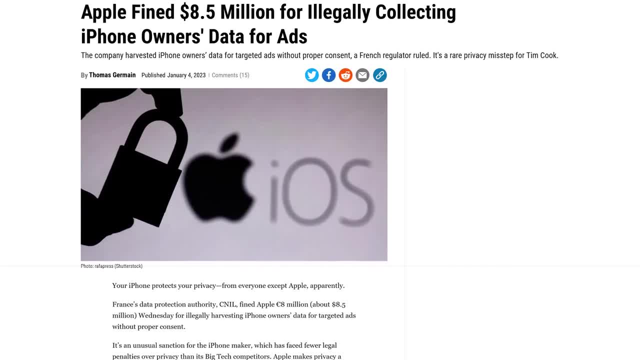 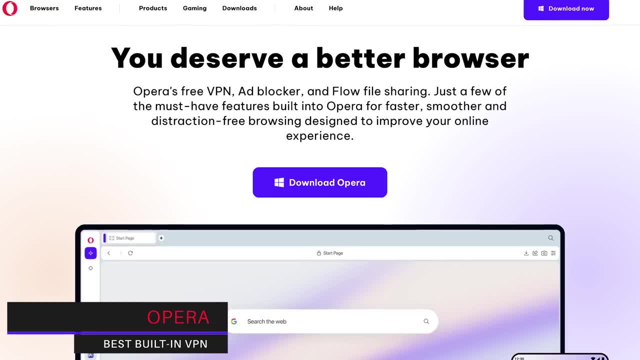 regulatory action being taken against them for not entirely being forthcoming with its users. Up next, Opera is the best for those of you looking for a free built-in VPN. To be technical, it's not a true VPN, It's actually an encrypted proxy server. 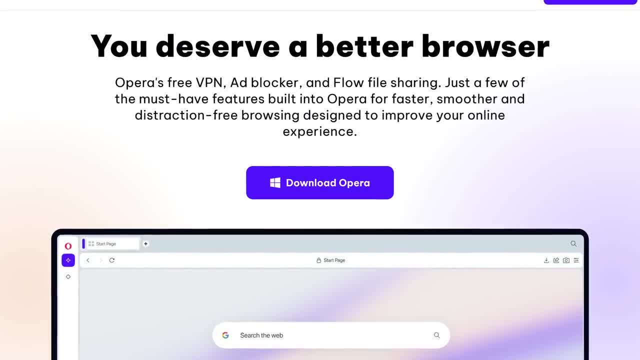 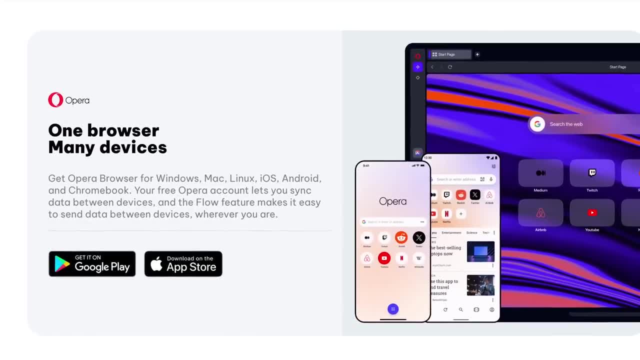 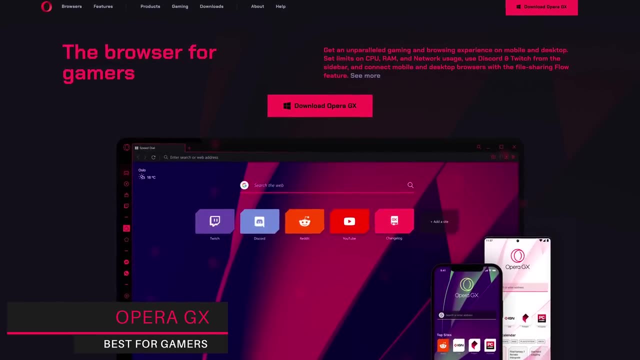 which can be useful to hide who you are and what you're doing online. Available for all the major platforms, Opera also includes a built-in ad blocker that also blocks crypto mining trackers and scripts. Another browser from Opera called Opera GX wins in the category Best Browser for Gamers. 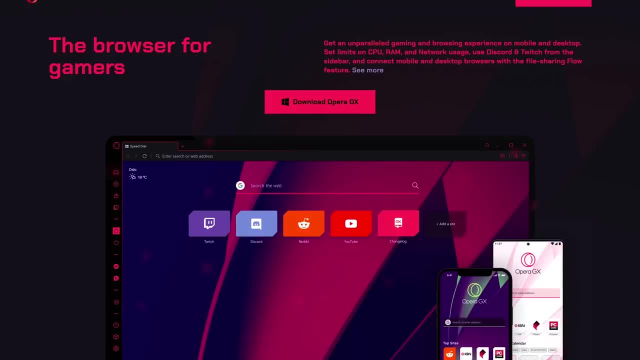 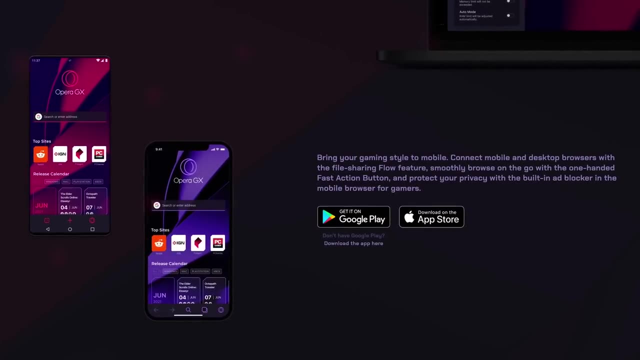 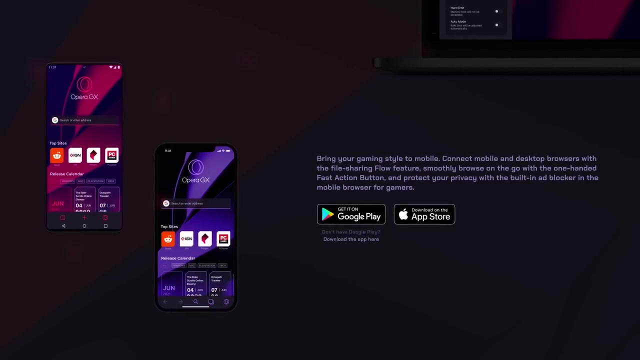 It has built-in features for gamers to help limit RAM, CPU and network usage, to help get the most out of both gaming and browsing. It also features integrations with both Discord and Twitch. Opera GX is only available for Windows, Mac, iOS and Android. At this time there's no. 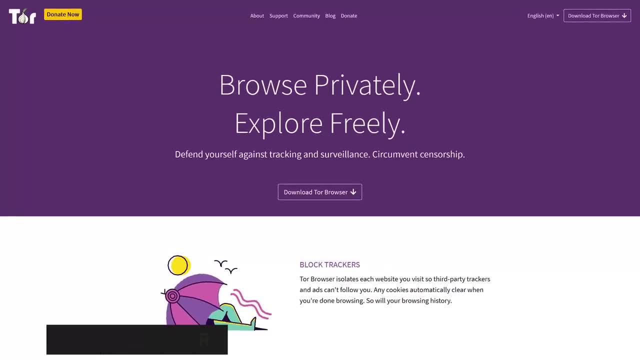 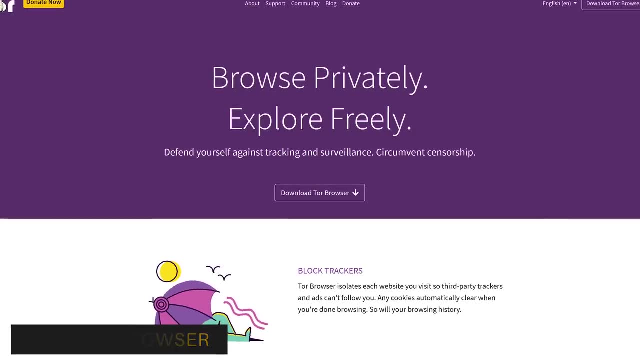 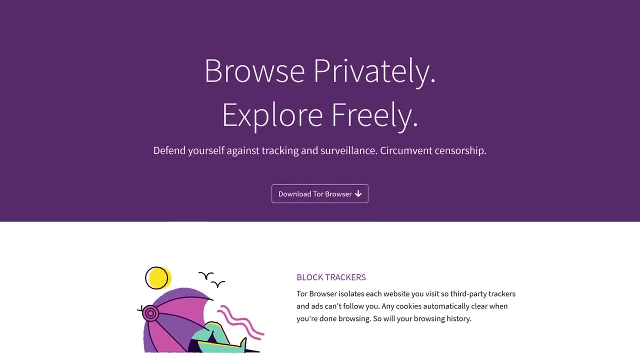 version for Linux. The Tor browser is the best to use to access the dark web, which is the encrypted portion of the internet that is not indexed by search engines. While the dark web gets attention for illegitimate activities, many companies and governments use it for legitimate purposes as well. 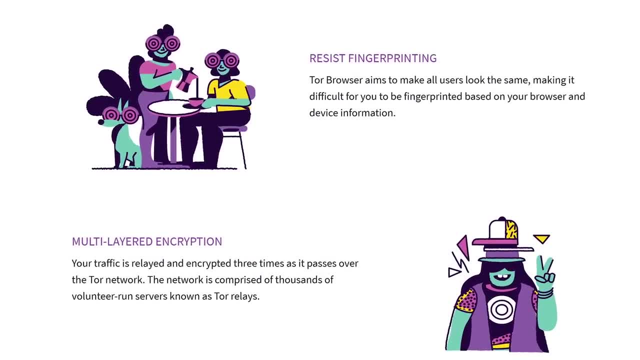 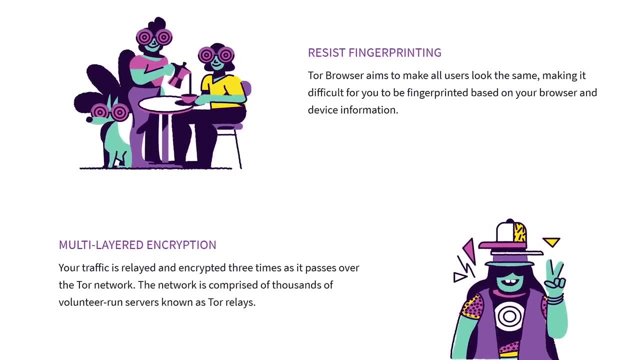 Using a modified version of Firefox. it also works to keep you anonymous while online through a network of more than 7,000 relays. Because of this, speeds are slower than all the browsers mentioned. The Tor browser is available for Windows, Mac, Linux and Android At this. 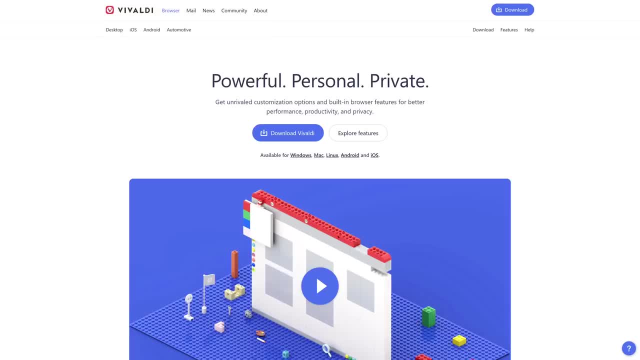 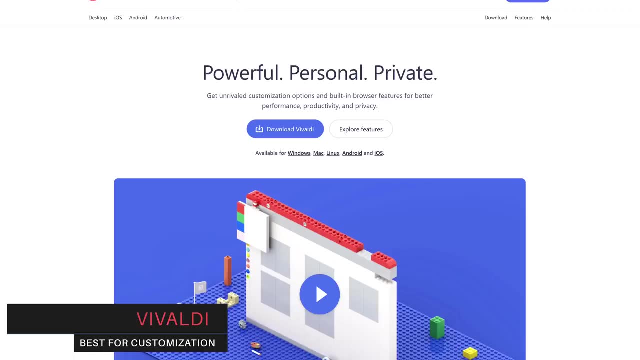 time it's not available for iOS. In the category Best for Customization, nothing tops Vivaldi. One of my favorites is created by one of the founders of Opera. It's great for those of you focused on productivity, with a ton of useful features. 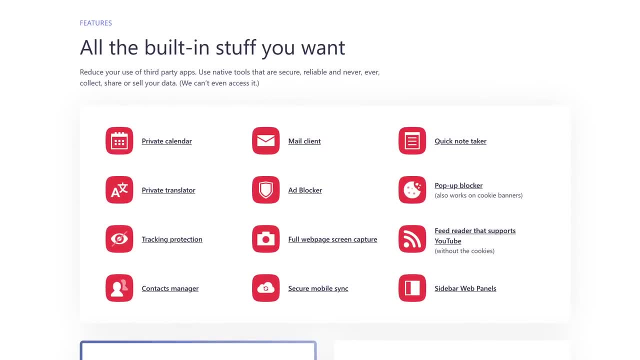 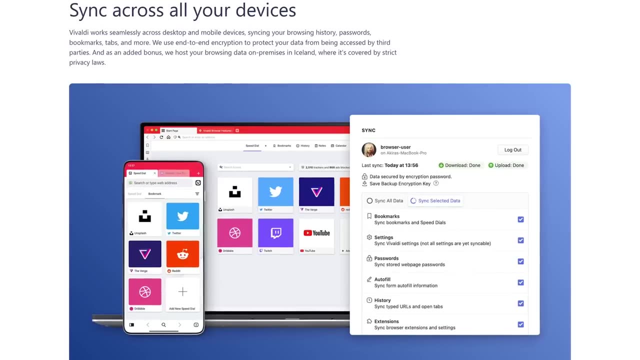 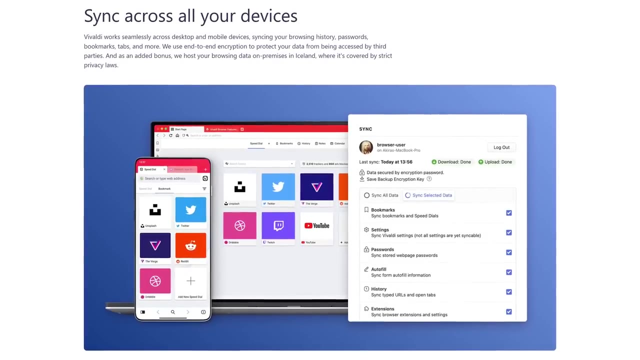 Some of those include an ad and tracker blocker built-in. It also includes its own email client, calendar and newsfeed. Having added a version for iOS this past year, Vivaldi is now available for all the major platforms to be able to sync your data with end-to-end encryption to all your devices. 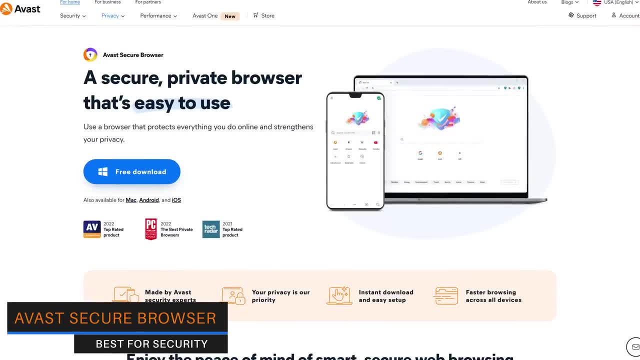 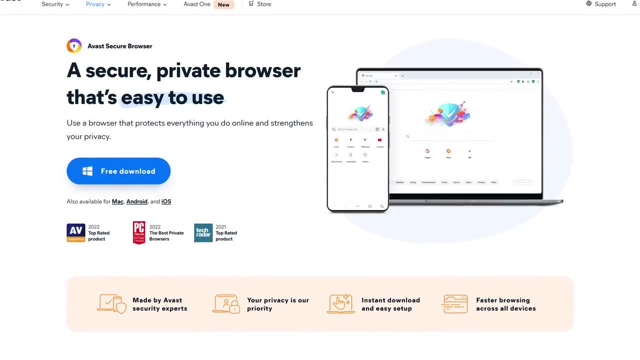 The best browser for security is one most people have never heard of: The Avast Secure Browser from the well-known antivirus company. Avast has tools built in to keep your data secure, while online There's an anti-fingerprinting and phishing module, ad blocker, tracker prevention.